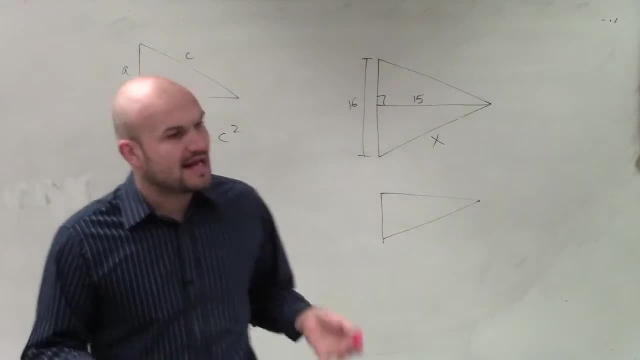 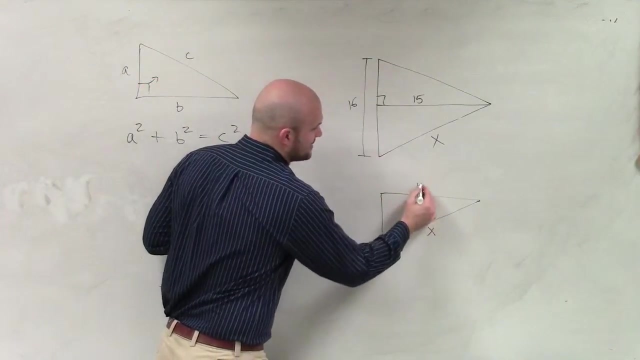 Flip that over, please, Thank you. So just to take that out and just focus on what triangle you're trying to work with. So we're just trying to work with this one. So the only thing I know right now is x and 15.. 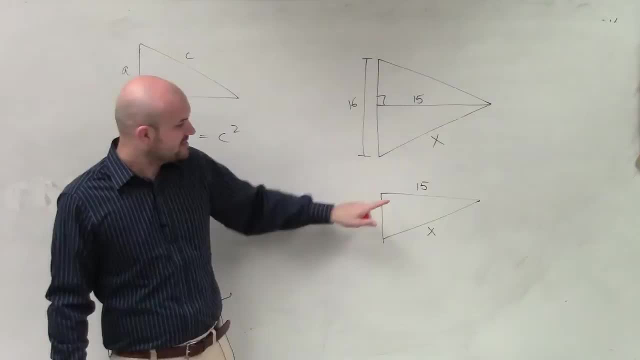 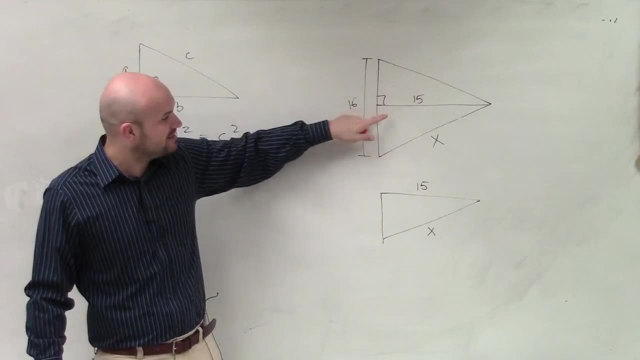 That's all I know right now. But now let's go and see. Can we determine this as a right triangle? This is a right angle. If this is a line and that's 90 degrees, can we assume then or prove that that has to be 9 degrees right? 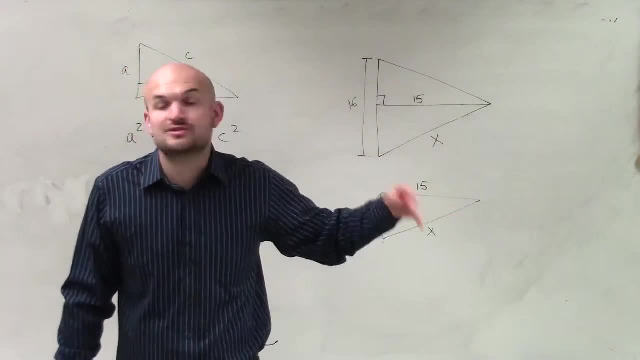 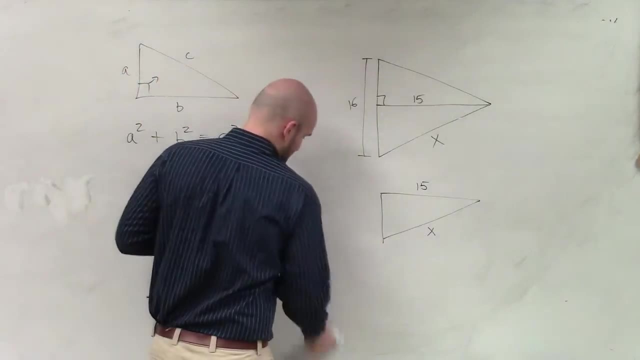 If it creates a line, then we know that's going to be a linear pair. right Where two angles make up a line are also supplementary, meaning they add up to 180.. So if one's 9 degrees, that means this has to be 9 degrees. 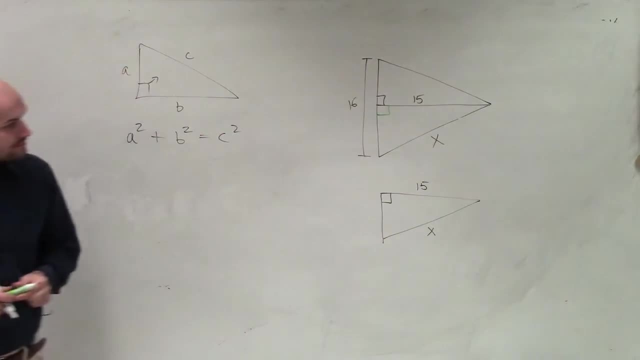 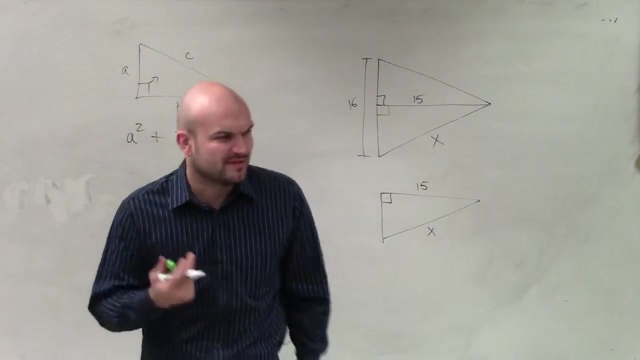 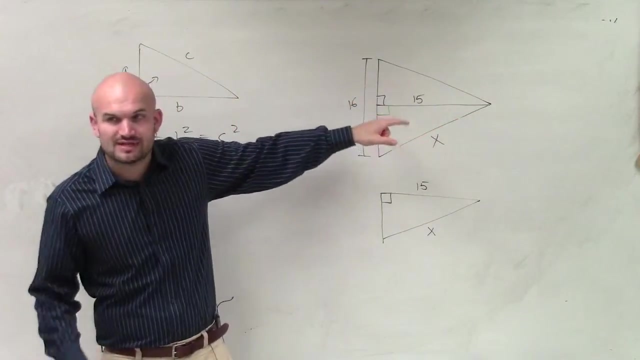 So, therefore, I can now show that that's 90 degrees. all right, All right. Where else was that? And I believe also this says that this is also going to be your bisector. This is your perpendicular bisector. I don't have the exact problem right in front, but it says this is going to cut this in half. 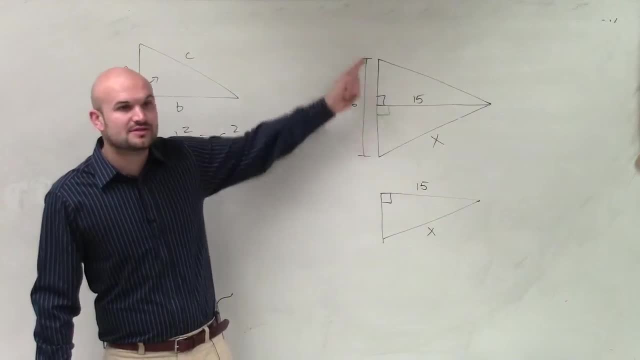 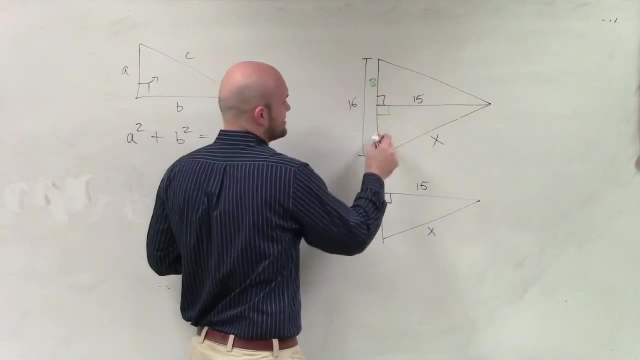 So if this whole side is 16,, what would you then assume? that both of these sides are going to be 8 and 8.. So now we can say that that's 8. And that's 8.. So now, ladies and gentlemen, 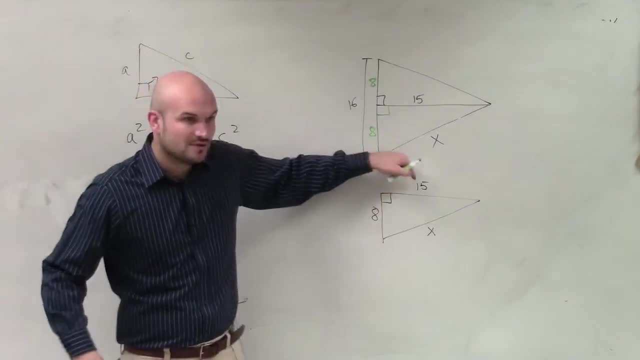 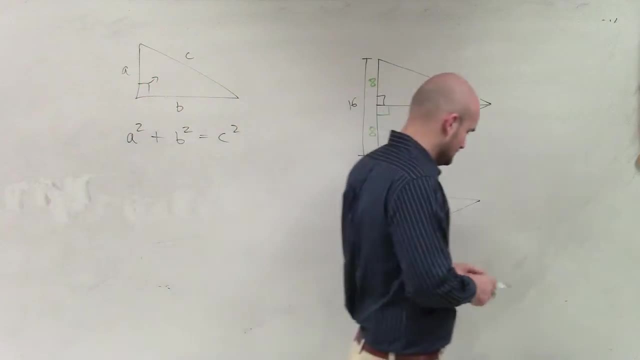 here's what we're going to see. Here's what we're going to see and, gentlemen, I can apply the Pythagorean theorem. I have two legs and a hypotenuse, OK, So now it's going right out the Pythagorean theorem. 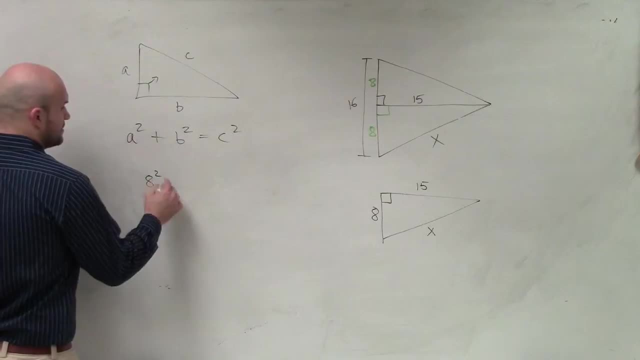 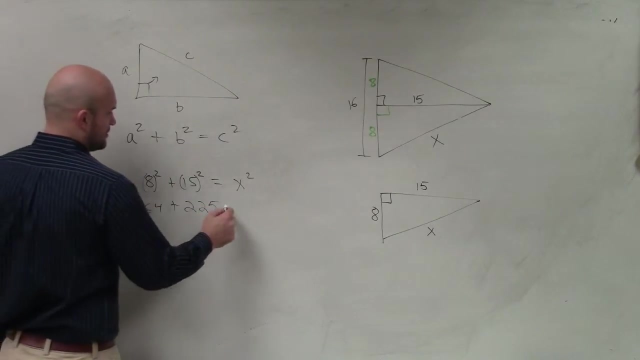 So in this case I have 8 squared plus 15 squared equals x squared. where x is going to represent my c, 8 squared is 64,, 15 squared is 225, equals x squared. Then I add those up together, so I have 289 equals x squared. 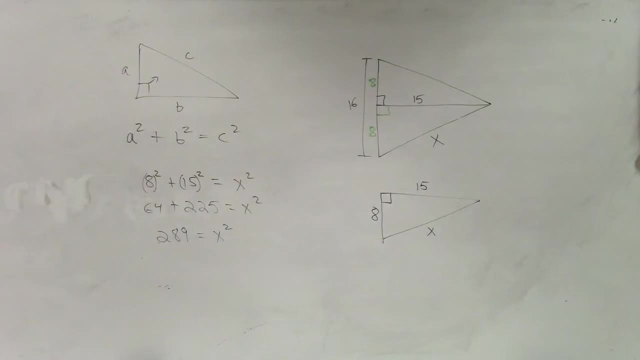 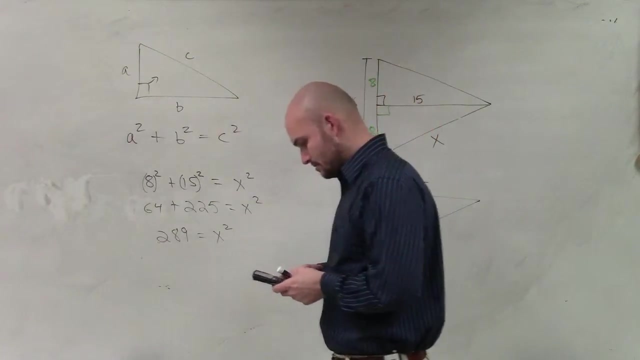 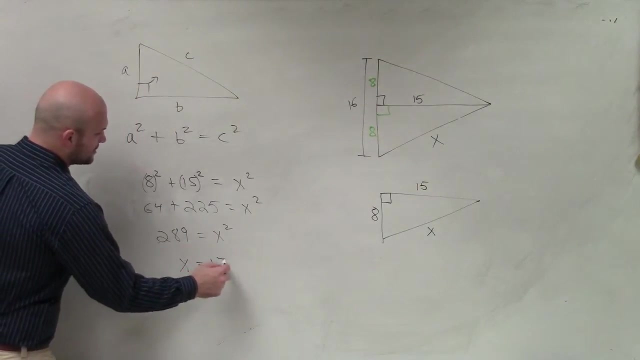 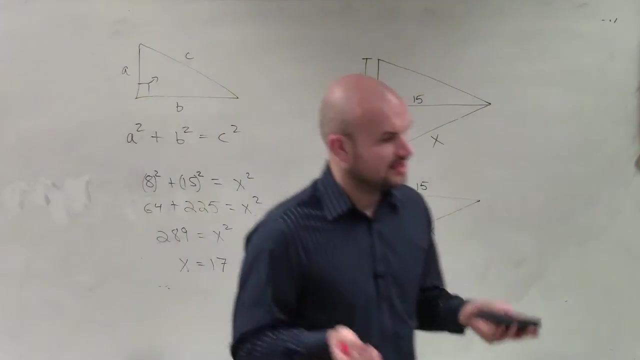 And see if I can simplify that any further. And the square root of 289 is 17,, which I did not have memorized yet. So x is going to equal 17.. OK Questions. That was your answer. I know I graded all those correctly. because I had a lot of 0's and 8's.